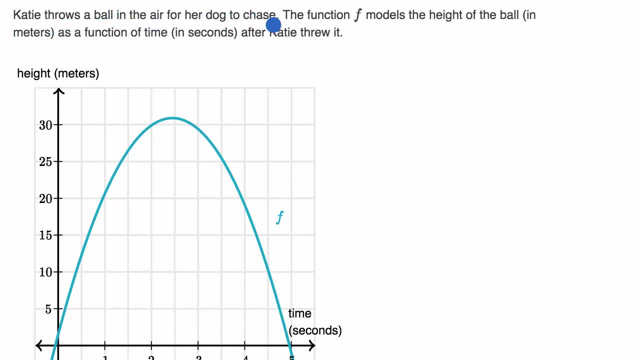 Katie throws a ball in the air for her dog to chase. The function f models the height of the ball in meters as a function of time in seconds after Katie threw it And we could see that right over here. This is our function f. 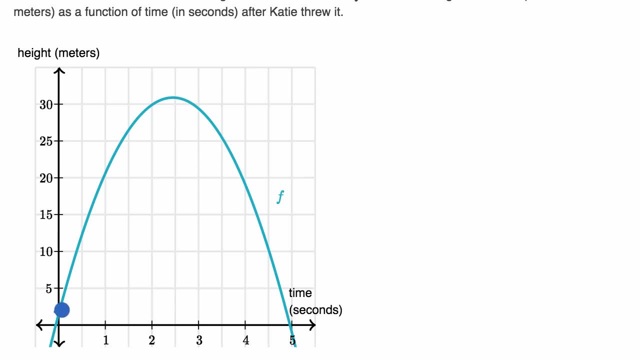 So at time t equals zero, the height looks like it's a couple of meters, And then, as we go forward in time to a little under 2 1⁄2 seconds, the ball's going up. And then, after a little under 2 1⁄2 seconds, 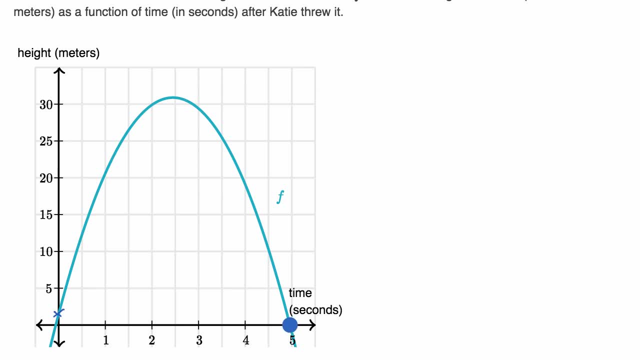 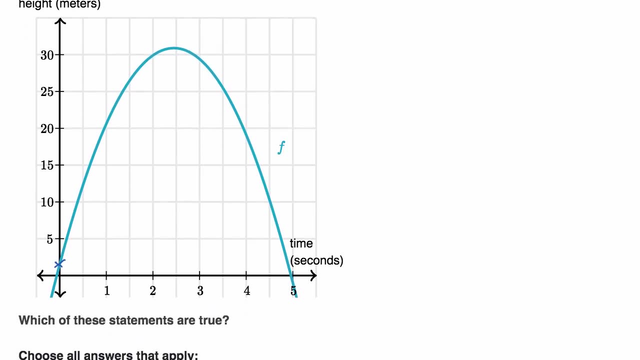 the ball starts going down, And by the time you get to five seconds, or close to five seconds, it looks like the ball is on the ground. Its height is zero meters. So then they ask us which of these statements are true? Choose all that apply. 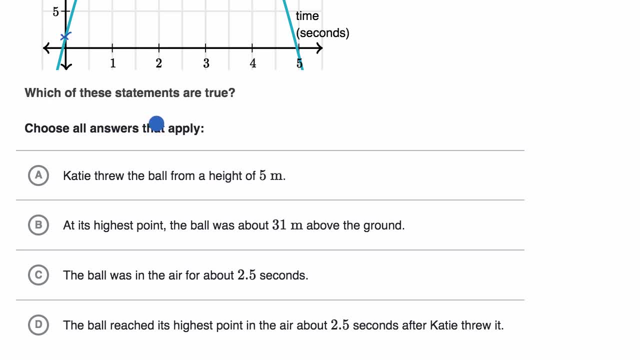 So pause this video and see if you can work it out. All right, now let's look through the choices. So the first one says Katie threw the ball from a height of five meters. So let's see if that bears fruit, or see if that's true. 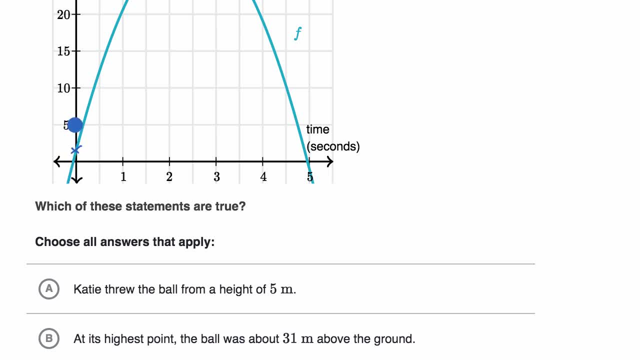 So if she threw it from a height of five meters, that means that the y-intercept would have been at five meters. At time t equals zero, it would have been at a height of five meters. Clearly that is not the y-intercept. 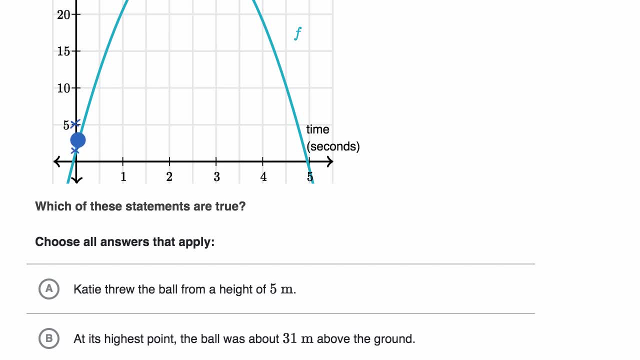 It looks like she threw it from a height of maybe 1 1⁄2 or two meters, So I'm assuming that Katie is not five meters tall, so she wasn't on a ladder or anything, She just threw it from her regular height. 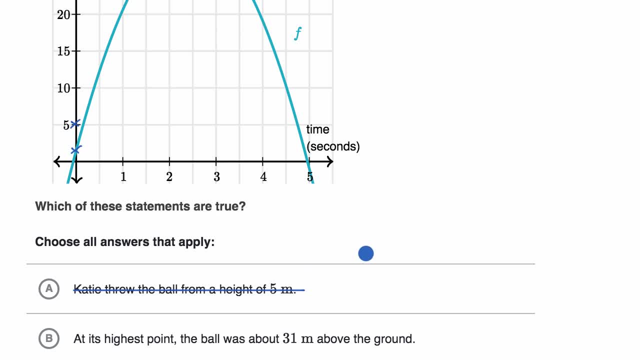 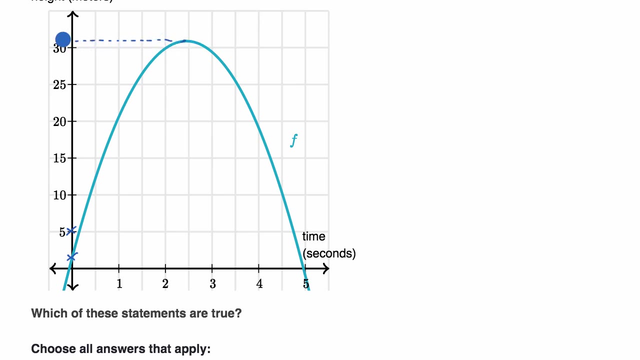 And so we can rule out this first choice. The second one says: at its highest point, the ball was about 31 meters above the ground. Let's see if that is true. So the highest point is right over here And, yeah, that looks about 31 meters. 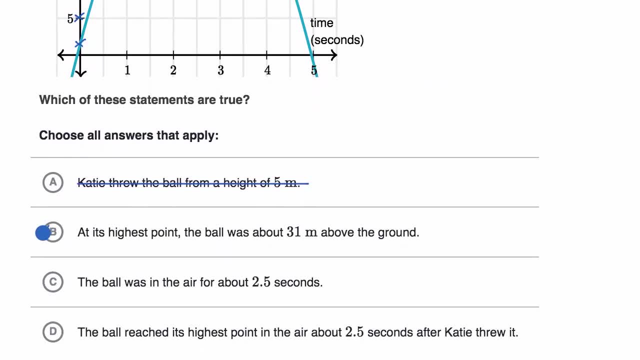 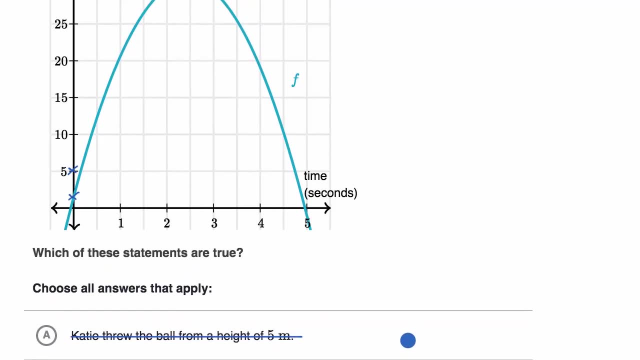 So I like that choice, So I will select that one. The ball was in the air for about 2 1⁄2 seconds, So we can clearly see that that is not the case. The ball was going up for about 2 1⁄2 seconds. 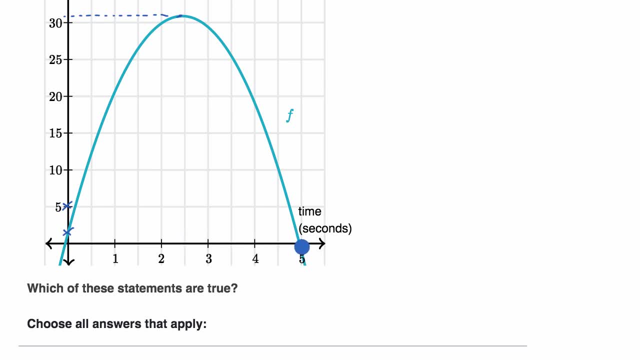 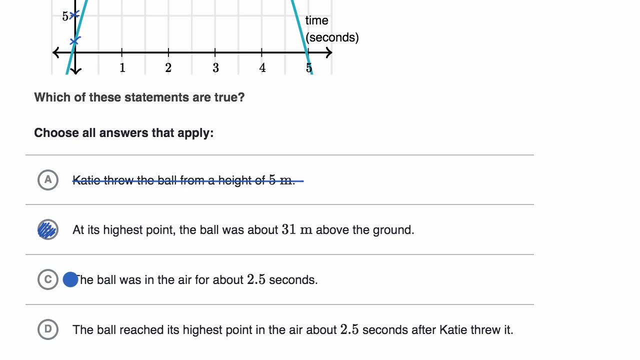 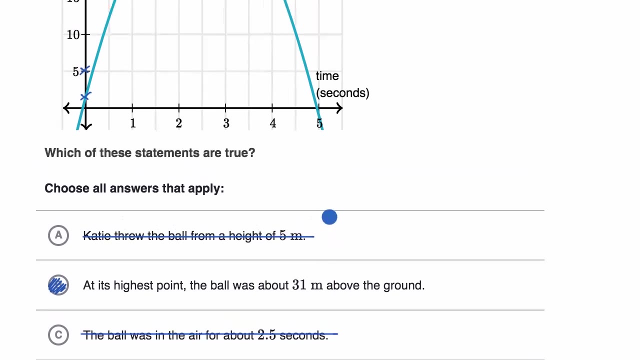 but then it was going down for roughly another 2 1⁄2 seconds, And so it was actually in the air for almost five seconds, So I would rule this one out. The ball reached its highest point in the air about 2 1⁄2 seconds after Katie threw it.